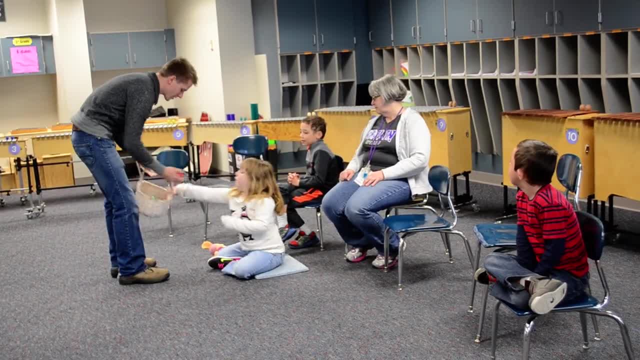 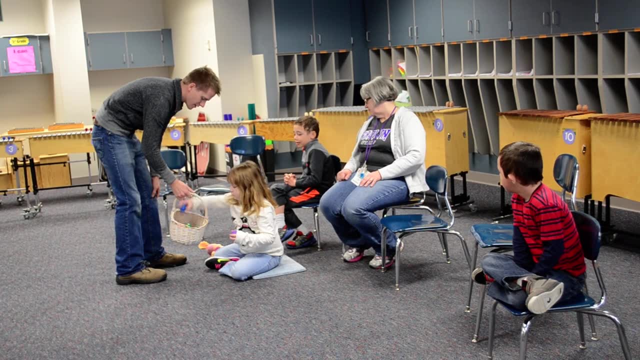 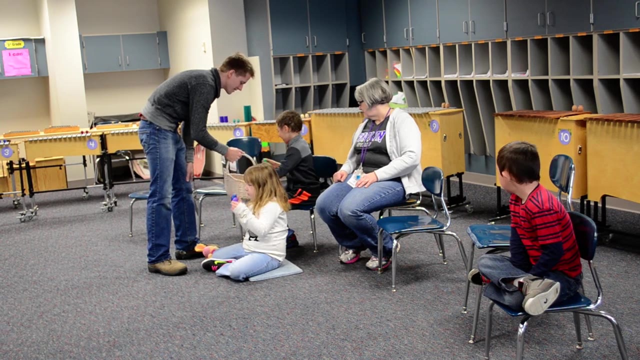 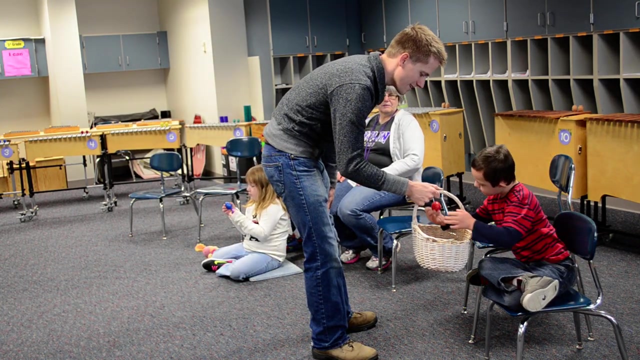 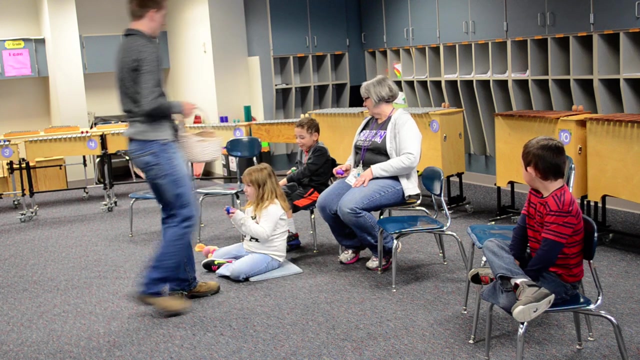 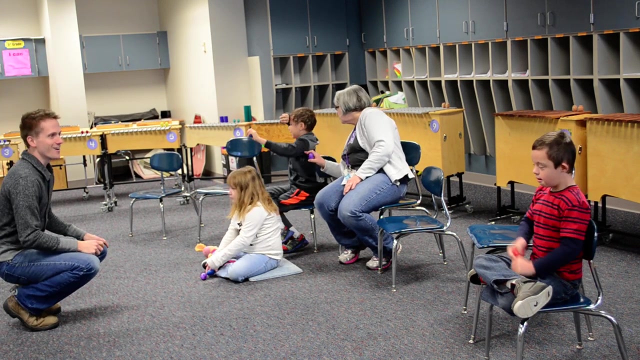 Well, good morning everybody. Today we're going to start with our good morning song, Thank you, Would you like to Hayley? Would you like to? Very good, Okay, now we're going to sing the good morning song. 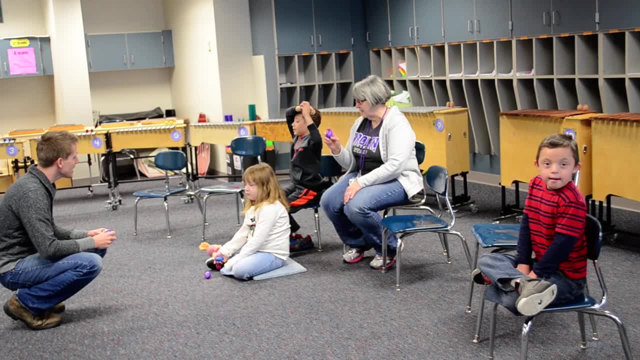 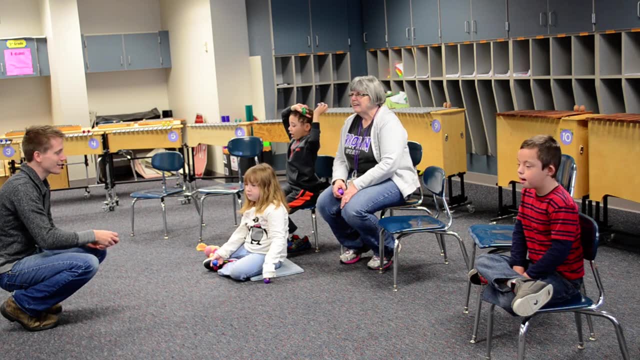 And what I'd like you guys to do is shake your eggs when it's your turn. So, Joe, I'm going to have you start, okay, Alright, here we go. Good morning, good morning, and can we play with you? 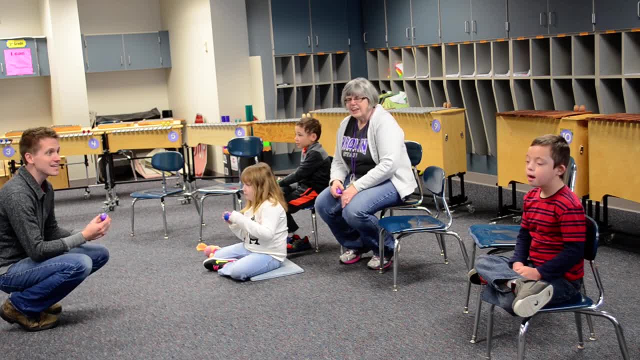 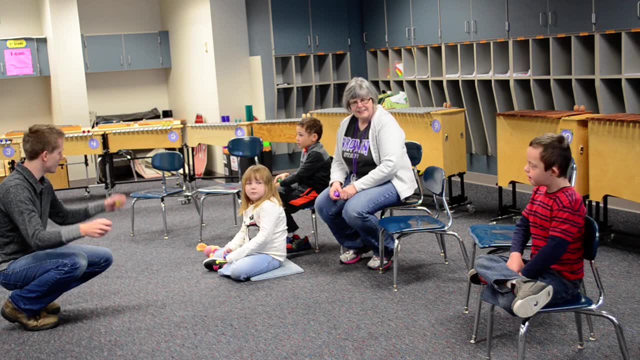 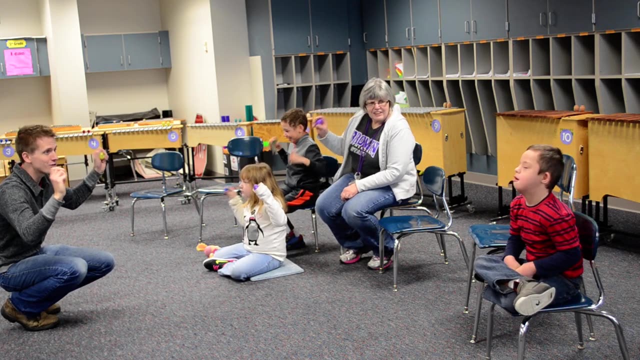 We're shaking, we're shaking, Shaking along with you. Now, Joe, how would you like to shake your shaky eggs? Very good, Can we all shake like this? Good job, Okay, let's sing it again: Good morning, good morning, and can we play with you? 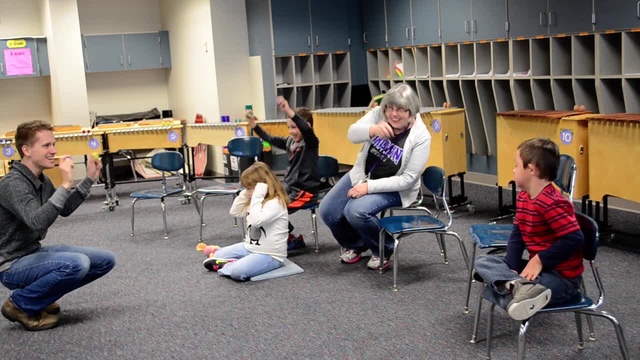 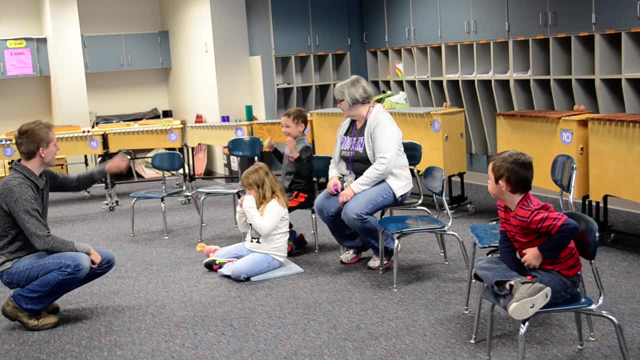 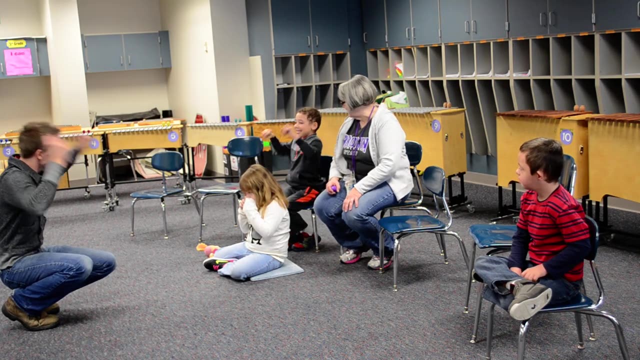 We're shaking. we're shaking, Shaking along with you. Thank you, Joe. Alright Miles, will you show us how you like to play? Can you shake? Ooh, he wants to shake them a lot harder, like this. 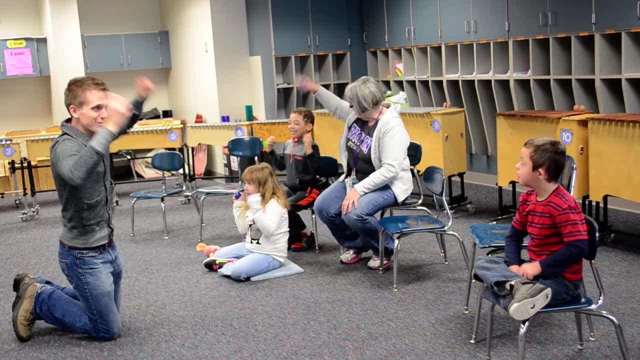 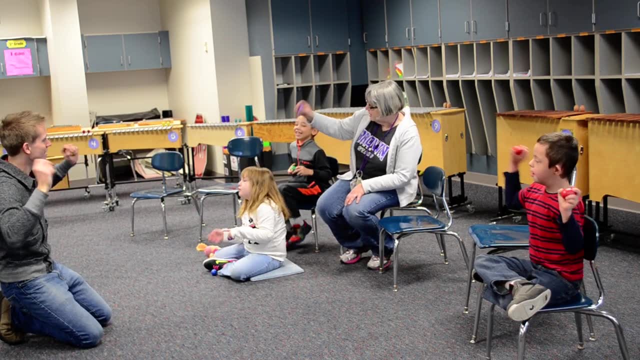 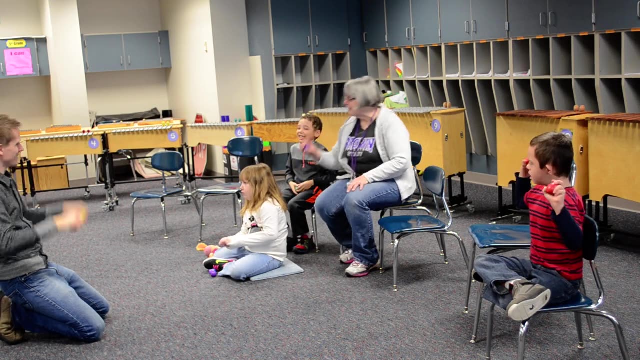 Okay, Hayley, can you shake like that? And Joe, will you shake just like that? Good, Good morning, good morning, and can we play with you? We're shaking, we're shaking, Shaking along with you. Okay, Hayley, it's your turn. 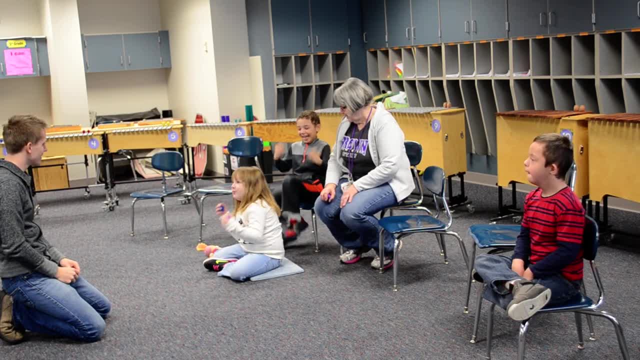 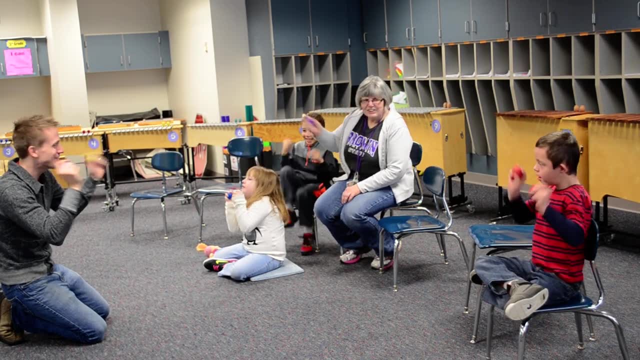 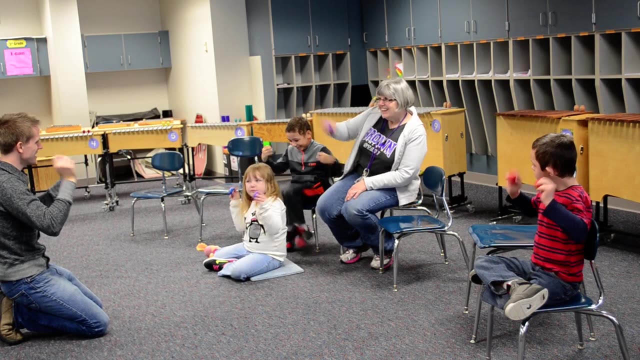 How would you like to shake your eggs? Good morning, good morning, and can we play with you? Good morning, good morning, and can we play with you. We're shaking, we're shaking, Shaking along with you. Good job, guys.